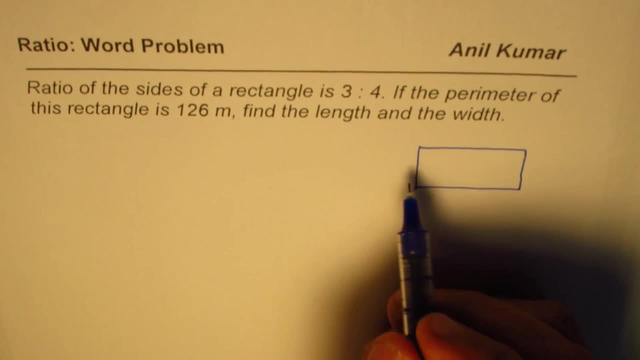 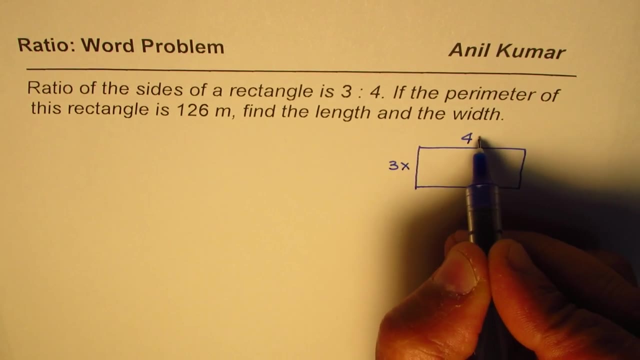 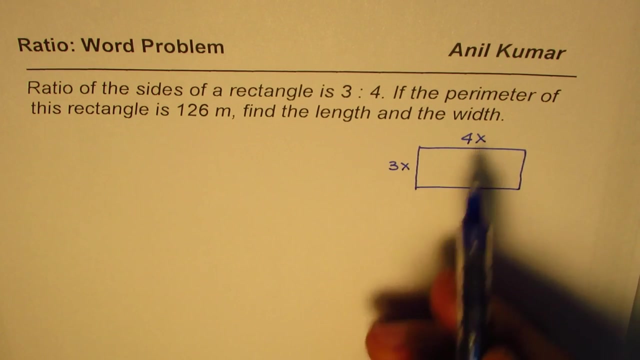 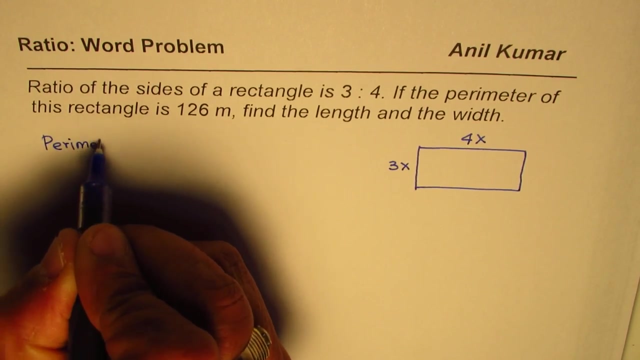 we are talking about has dimensions- width and length- in the ratio of 3 is to 4.. So we could say: 3 times any number is the width and 4 times any number is the length. Then the ratio will be 3 is to 4.. We are given that the perimeter is sum of all the sides. 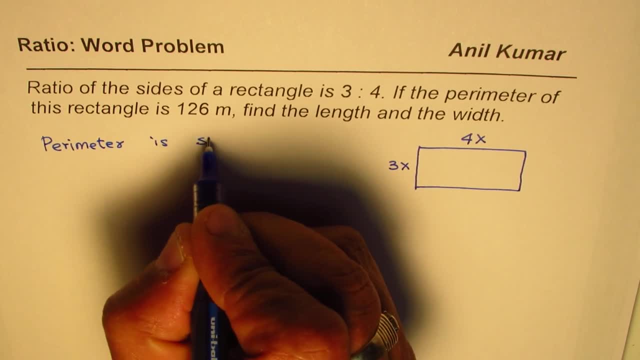 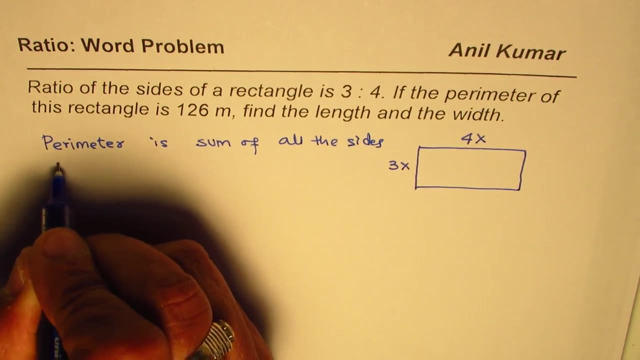 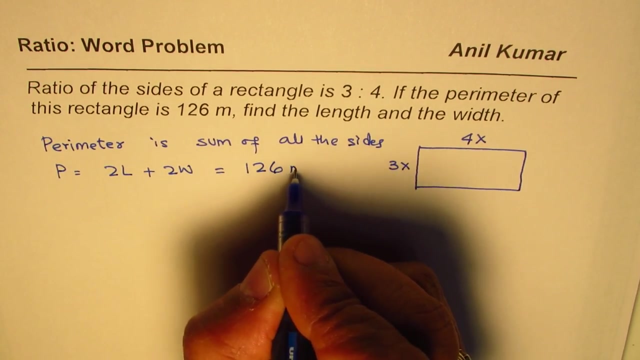 So perimeter is sum of sides, All the sides. So we say perimeter P is 2 times length plus 2 times width and that is given to us as 126 meters. We have to find what should be the dimensions or what should. 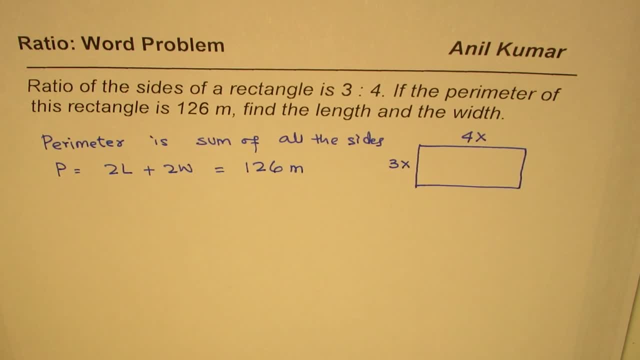 be length and width of this rectangle? That's the question for you. I hope the question is very clear. You can now pause the video, answer the question and then look into my suggestions. Now my approach is that we have already written perimeter. That means twice length and twice. 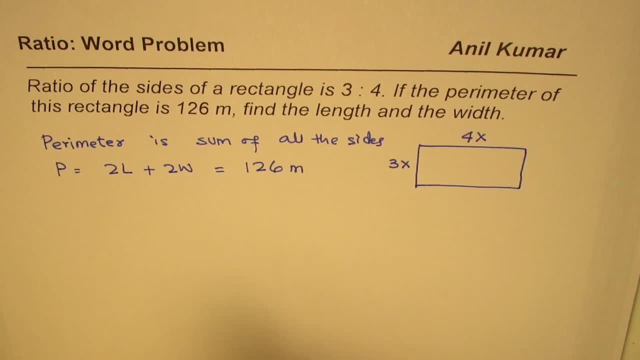 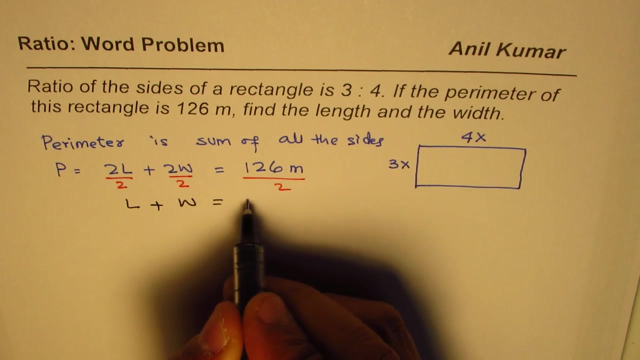 width is 126.. Now, if I divide each by 2,, if I divide each by 2, right. so only adding length and width once, in that case I get: length plus width is equal to 12 divided by 2, which is 63, right? So that is the length plus width, 63.. 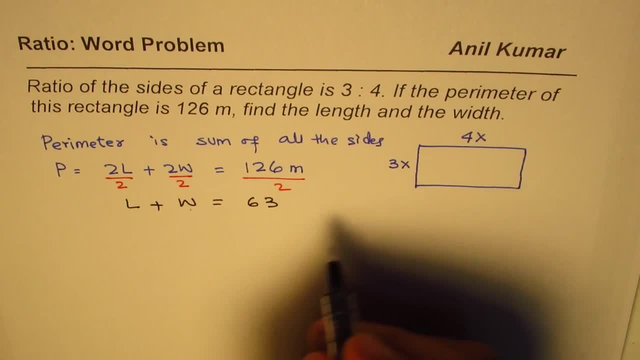 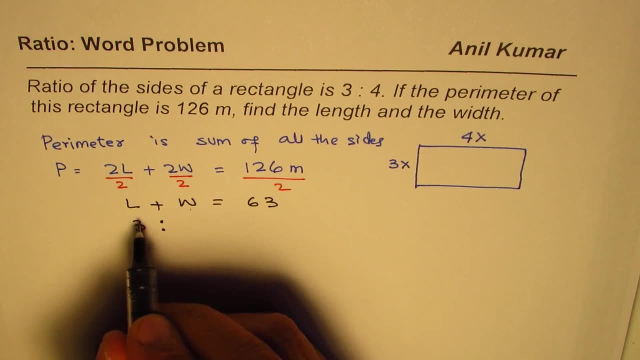 Now what we have here is the ratio of. we have ratio of length and width. is 3 is to? I mean because length is normally more. Anyway, 3 is to 4 is the ratio. At the end we'll change length to be a longer sign. Now, if the ratio is 3 is to 4, you also see 3 plus 4 is how. 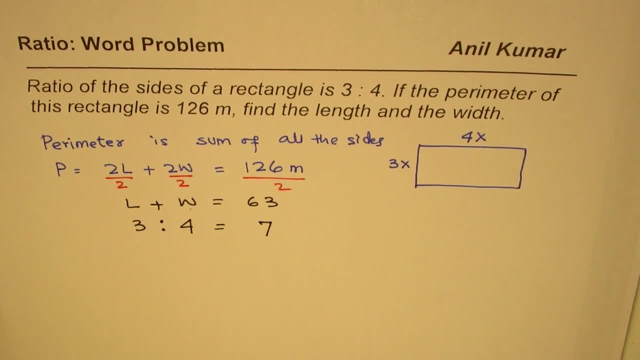 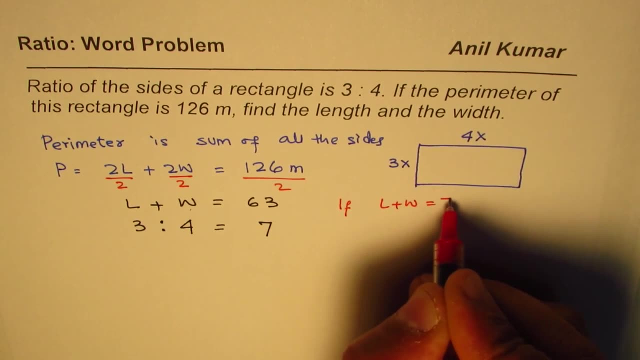 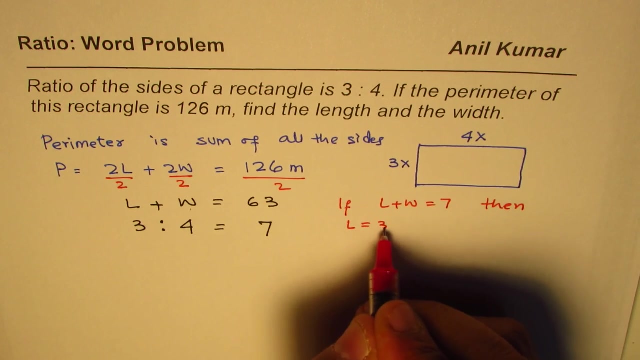 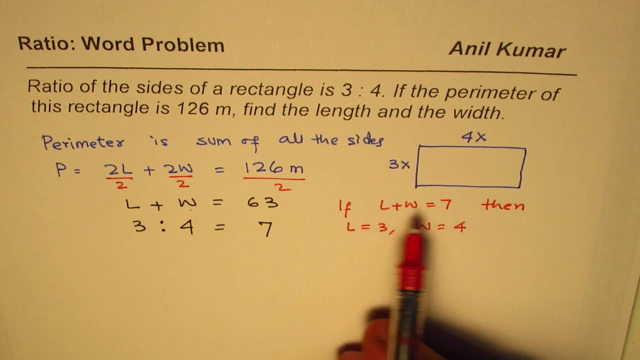 much: 3 plus 4 is 7.. That is to say, let's try to understand this- If length plus width equals to 7, then length equals to 3,, width equals to 4, correct? That is what we are trying to say, right? In our case, what do we have? We have length plus.